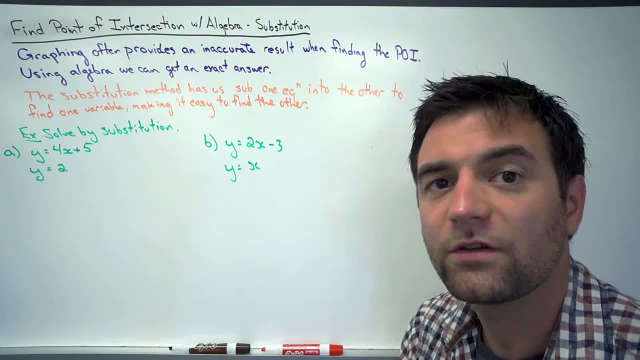 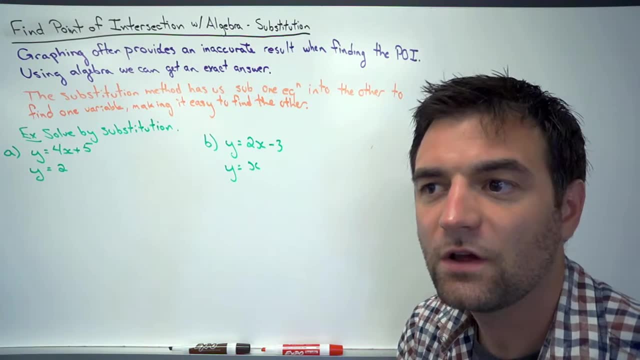 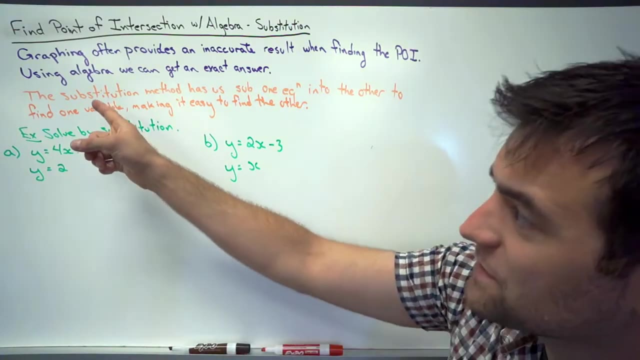 be just a little bit off and, depending on your graph, you could be off by a factor of five or six points to five or six hundred points, depending on the scale of your equations. So we like to use algebra, because we can get exact answers with algebra. Now the substitution. 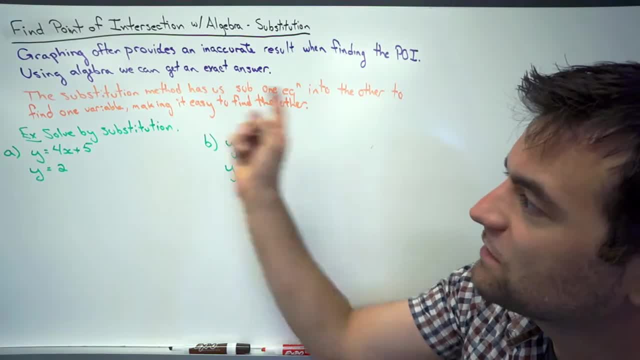 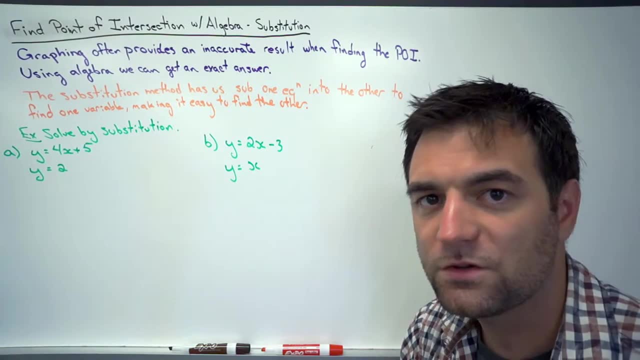 method. what it has us do is it has us sub one equation into the other to find one variable, and then it becomes very easy to find the remaining variable. So we'll look at a few examples and see the procedure in substitution. So in this first question here we have y. 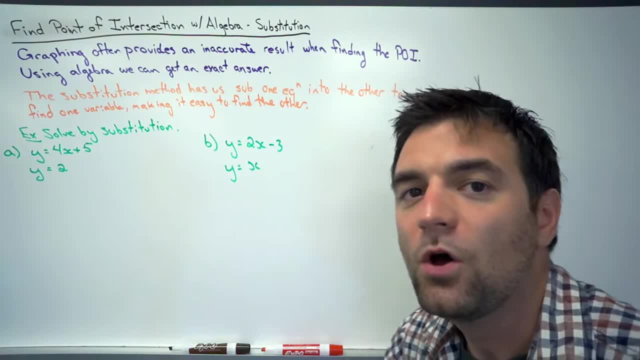 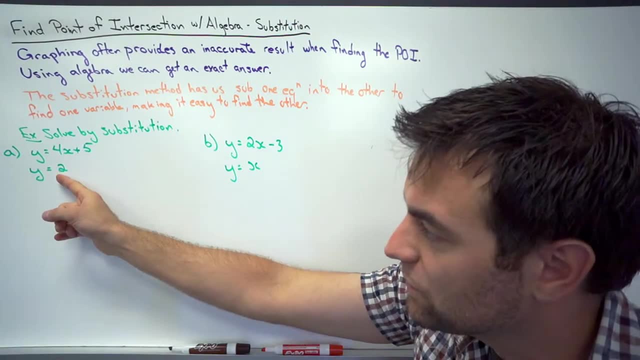 equals four, x plus five And y equals two. Here we have two different equations and I've set it up so that it's a little more familiar. The y equals two can be subbed in for the value of y, So if y equals: 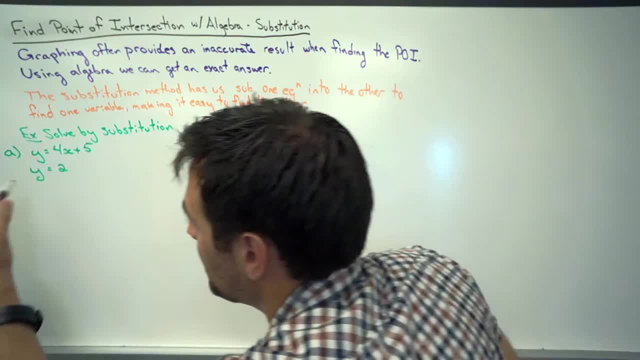 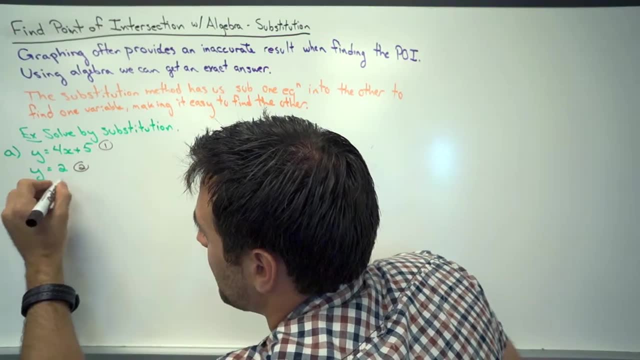 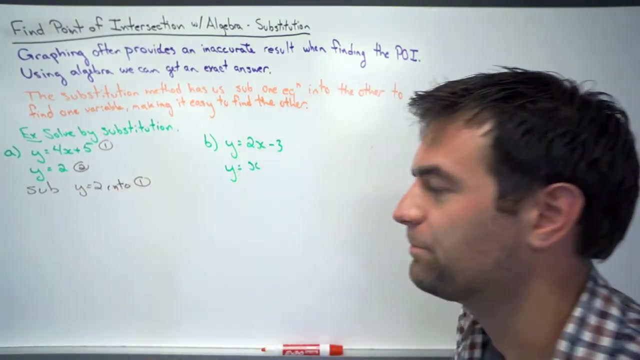 two. we could put that in for y. So I'm going to call this equation one and equation two and we're going to sub y equals two into equation two. So we just replace the y with the number two and we're going to use a different color. 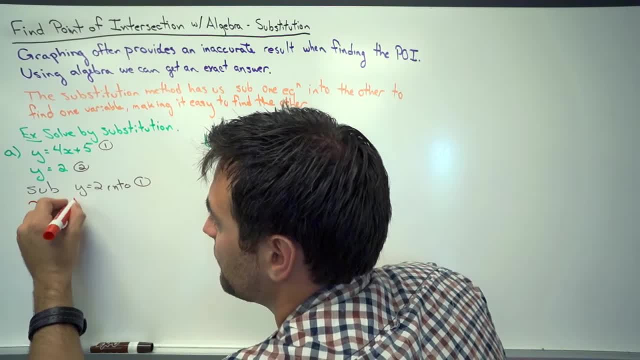 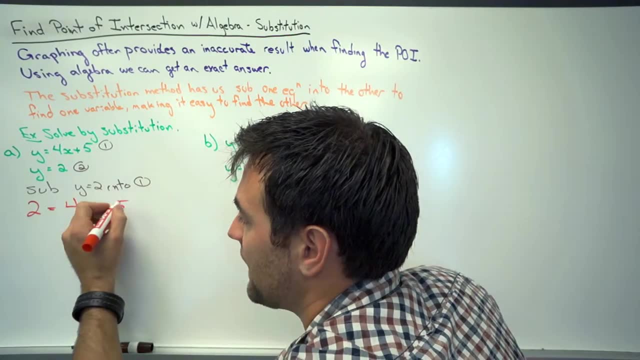 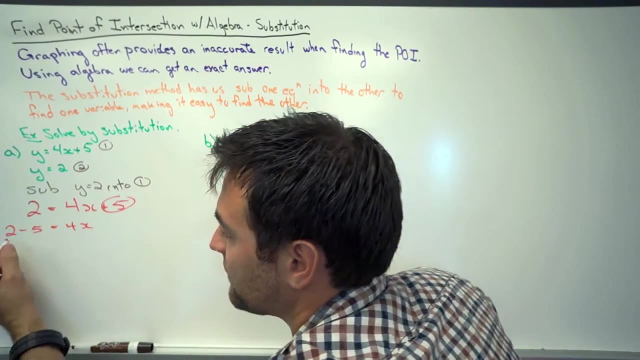 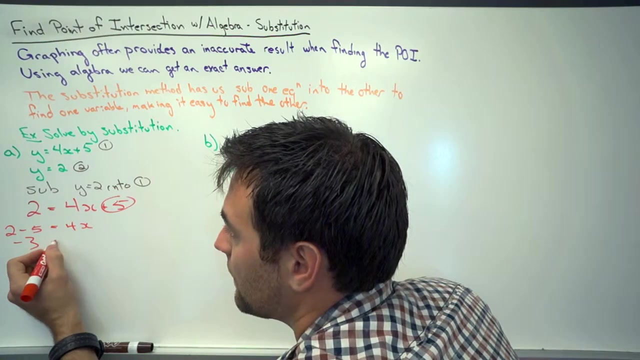 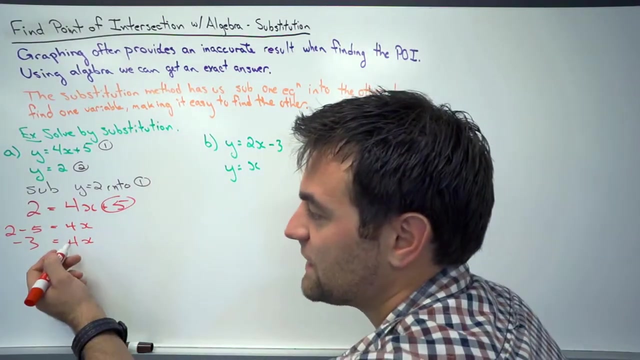 here: Two equals four x plus five. And now we go about solving this for x, So we'll move the five over. It'll become two minus five equals four x. Two minus five is going to be negative three, And then that equals four x, And then, to get the last part, we can take that four, move it over. 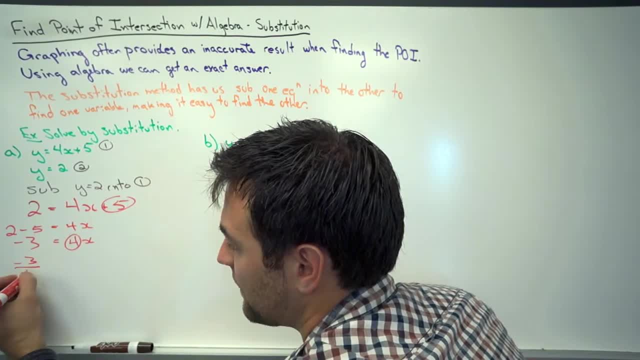 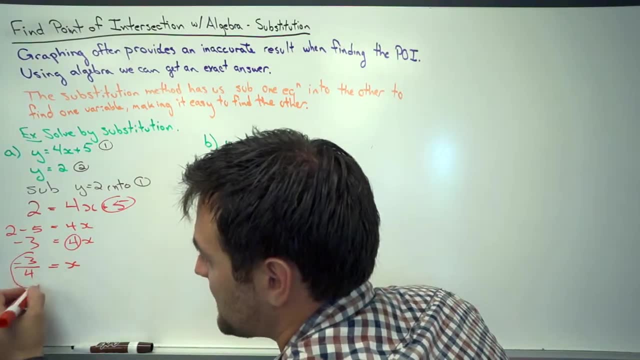 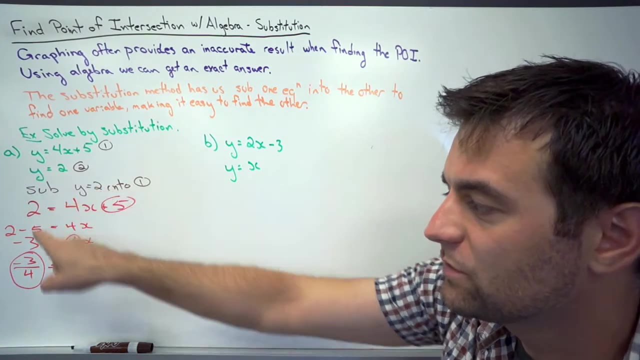 and divide. So we have negative three divided by four equals x. Now here we have a fraction as our value for x. So this is the x coordinate of the equation. We already know that y equals two and we have x equals negative three over four And 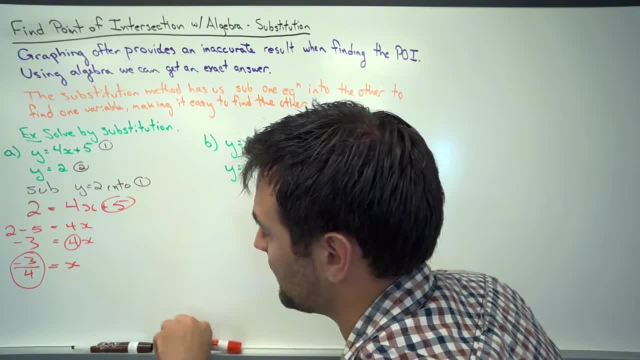 we're going to take the last fraction of that and all of the rest. So I'm going to start by adding a new hand. So I'm going to add a new fraction of the equation Here. we're just going to do what I showed you five times. We're going to add a new. 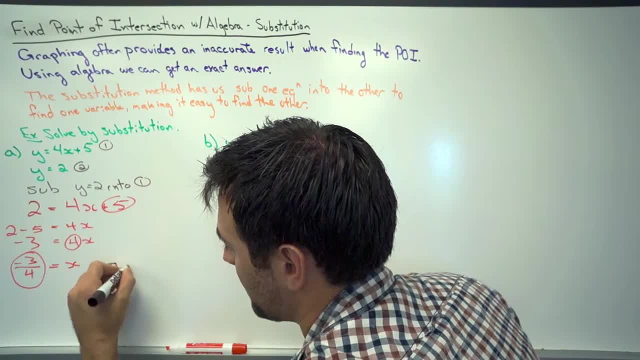 fraction for x. So we get you know whatever x equals four, And then we're going to add the next one, to add the next one to our equation So that the first one is a four point intersection. So again we're looking at the relation between x and five. This is just to make sure that I know what I'm going to do here. So what I'm going to do is I'm going to keep going with my equation. We're just going to add a new fraction that I want to add to this situation. 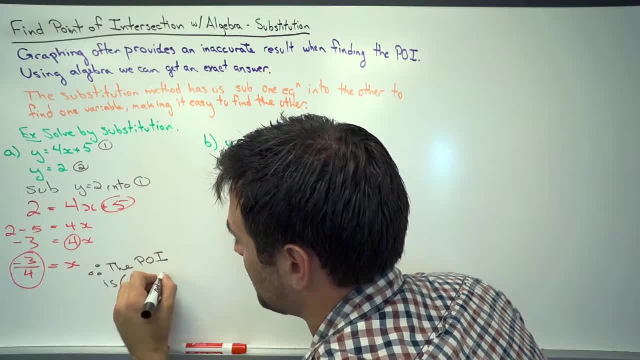 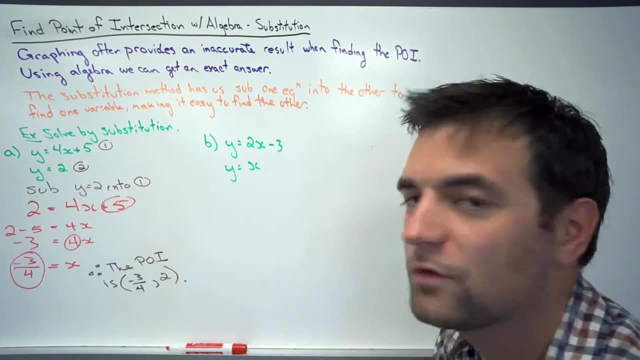 And we're going to add a new fraction to it that we just added earlier: three over four and two. So there's our x value that we calculated, there's our y value that we already know. So, once we have an x equals or y equals, 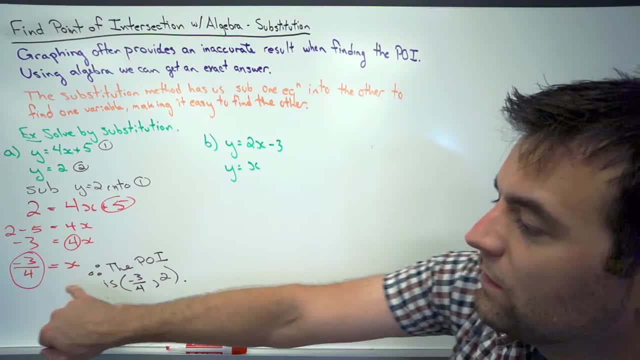 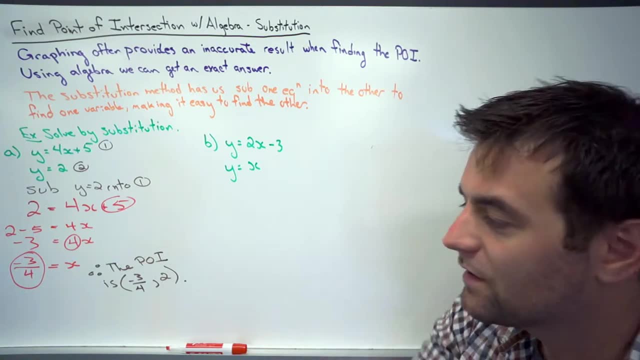 we're done finding that variable. This is through negative three quarters. this is a fraction. it's partway between two points on the graph. We couldn't get an exact answer like that easily on the graph. We think it was three quarters, but maybe it's not. 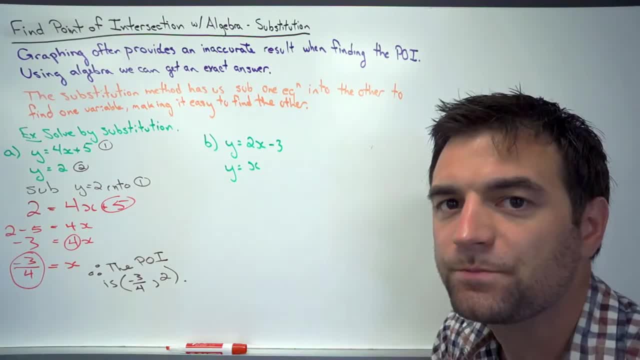 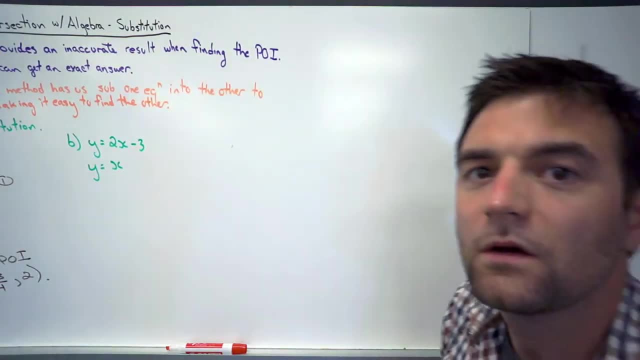 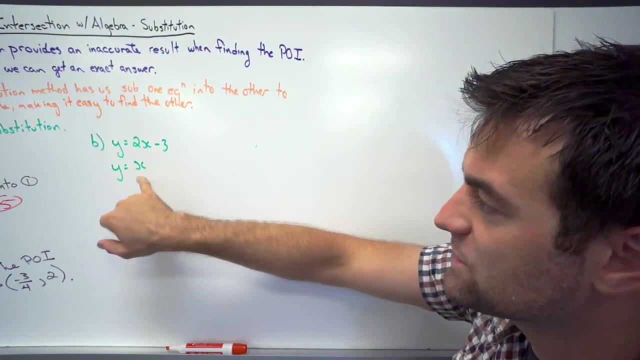 Maybe it's a little bit more, maybe it's a little bit less. Here we know it's exactly three quarters. Let's take a look at another example. So this is a little bit different. now We're doing substitution, but here we have y equals two, x minus three. 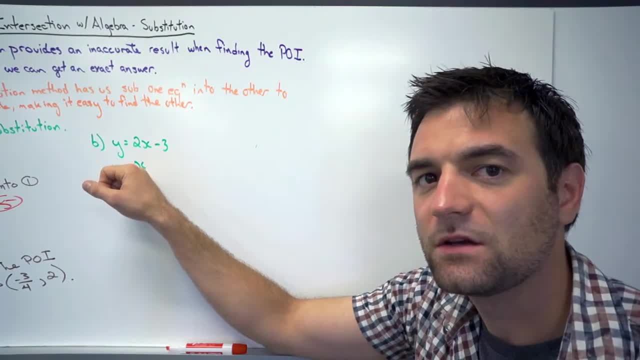 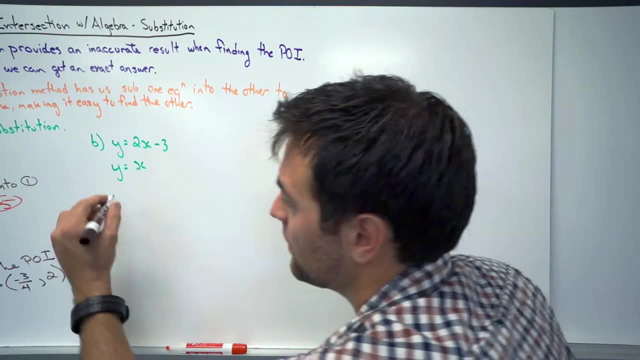 and instead of y equals a number, we have y equals x. So now we have a letter that we're gonna have to substitute in. It's done exactly the same way as the numbers, though We're gonna call this equation one and this equation two. 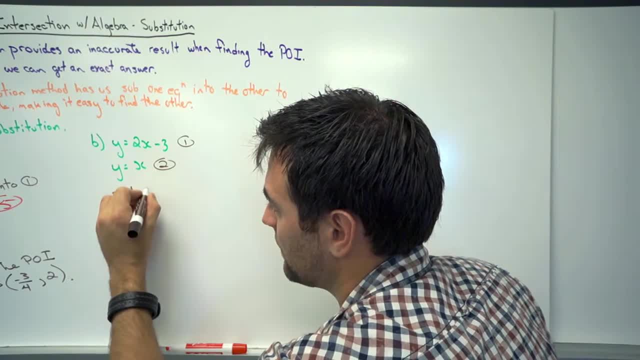 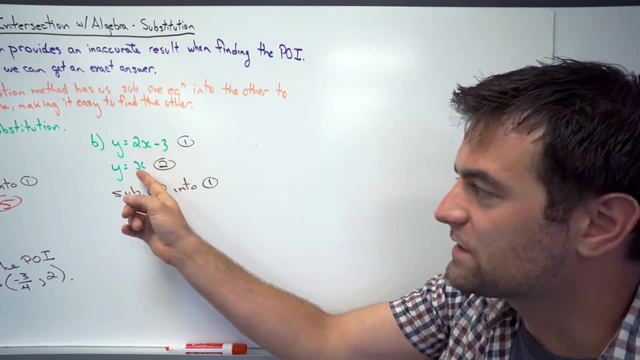 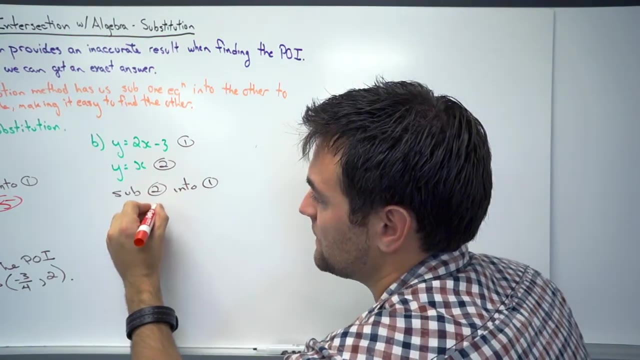 And I'm gonna sub that equation two into equation one again. So y equals x. so I'm gonna replace the y with the x. So x equals two x minus three. So I've replaced that y value with the value that y is equal to. 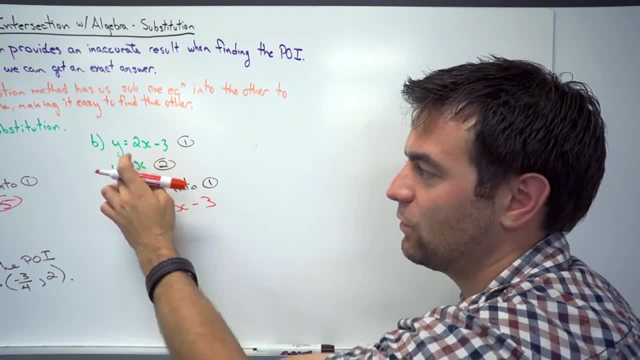 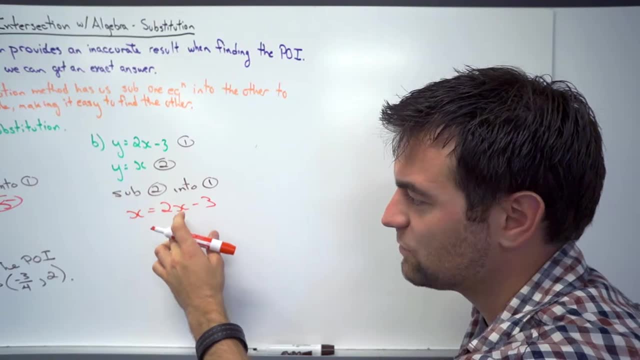 Y is equal to x. it's the same, so I replaced it. Y was replaced with the x, And now I go about solving this, So I already have an x on this side. I'm gonna move this two x over to that side. 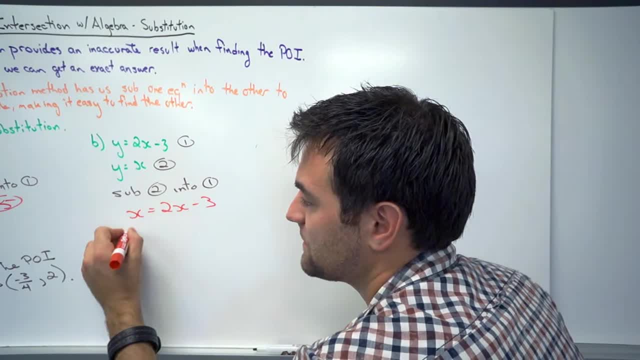 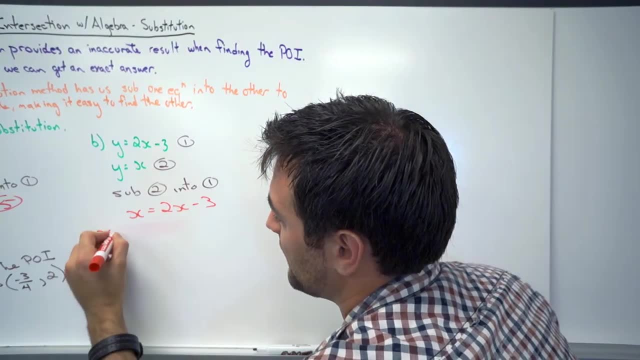 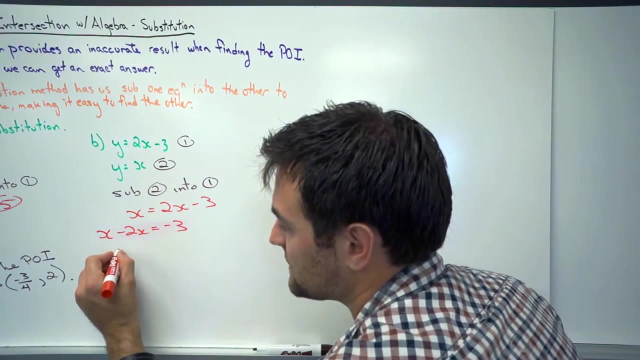 so I can get all my x's on the same side. So I have x minus two x. I'm gonna just rewrite that a little bit: X minus two x equals negative three. Now, x minus two x, that's negative one x or negative x. 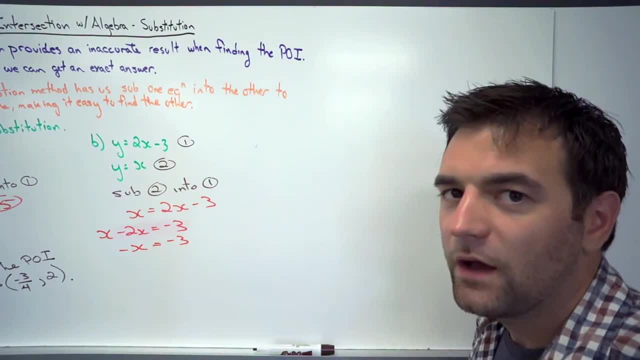 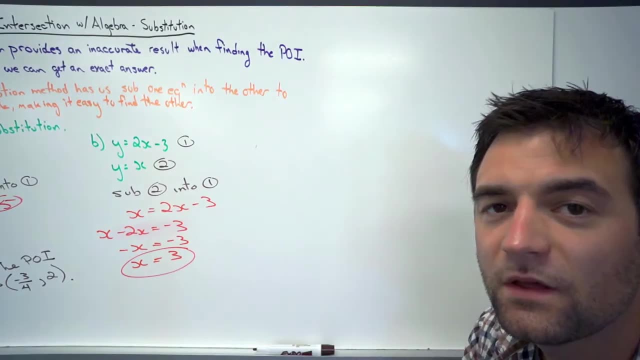 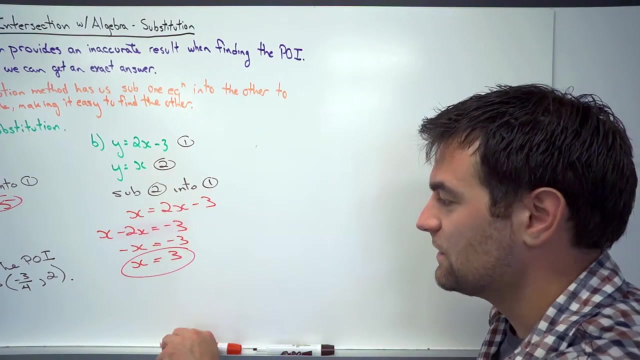 So negative x equals negative three, And now I can get x equals positive three. So there's my x value. Now, in this case, I'm not done. I don't know what y actually equals, yet I know y equals x, So what I need to do is take this value. 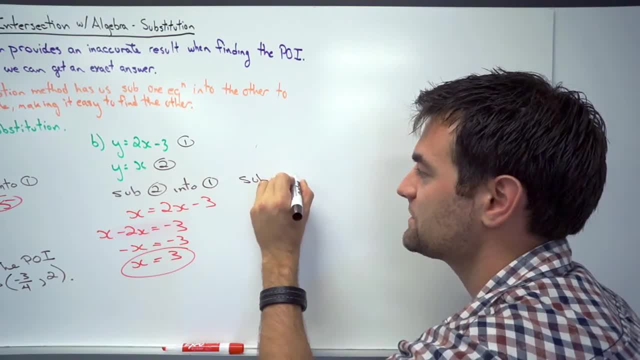 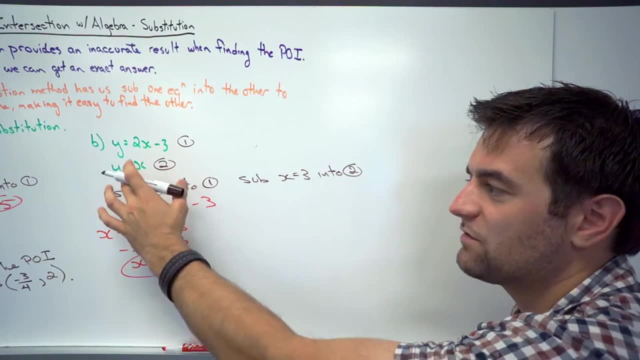 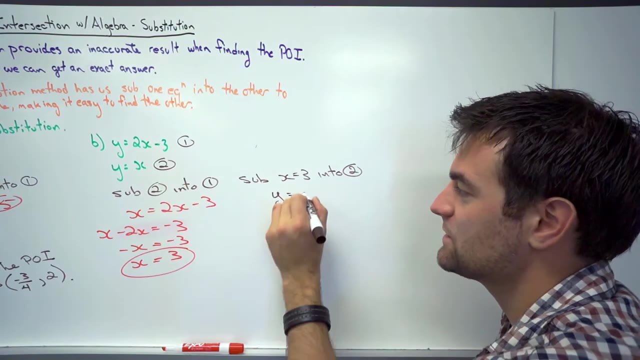 and sub x equals three into equation two. So I'm gonna sub it into this equation and find out what y is actually equal to. I know, when x equals negative three levels, I will do whatever I do, So'll take this point of intersection. 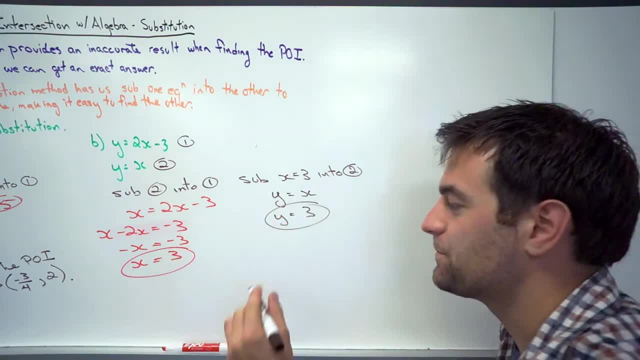 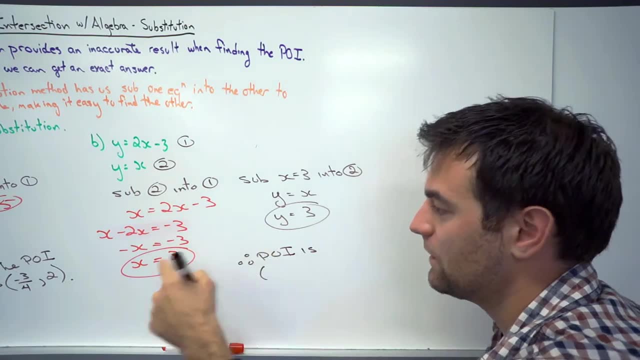 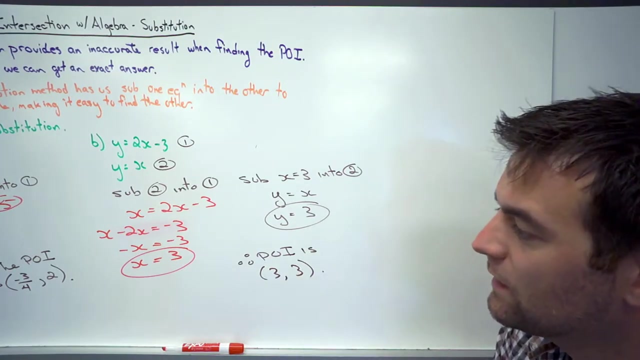 So y equals now x is three, so y equals x. that means y equals three. Now I know my x value and my y value. I know both values. I got that result. Therefore, the point of intersection x- y, 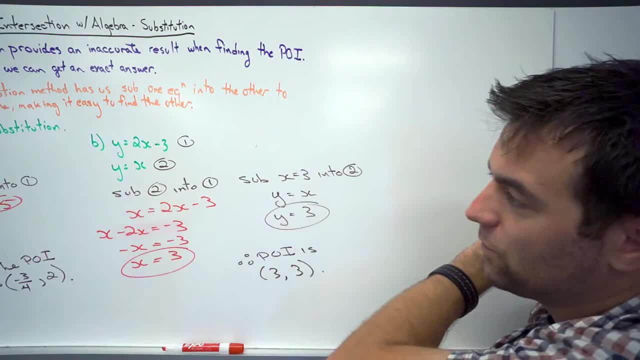 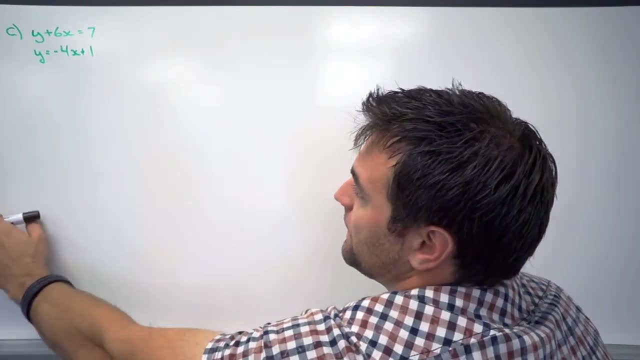 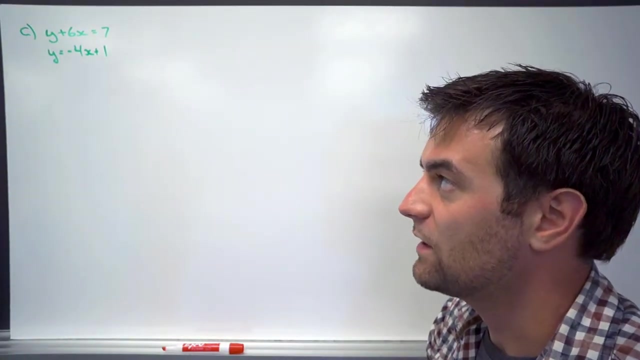 So the point of intersection is the x- y. further elaborate, we're going to make this a little bit tougher And here we have an example where y plus 6x equals 7 and we have y equals negative 4x plus 1.. 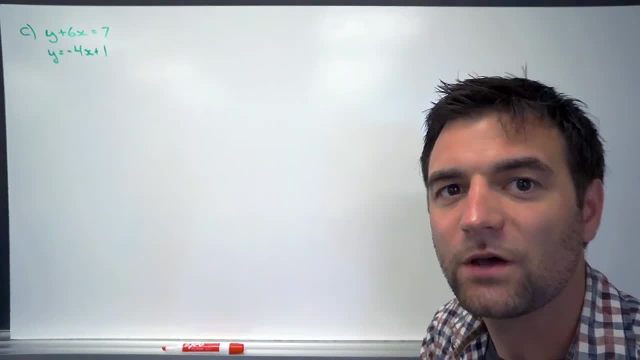 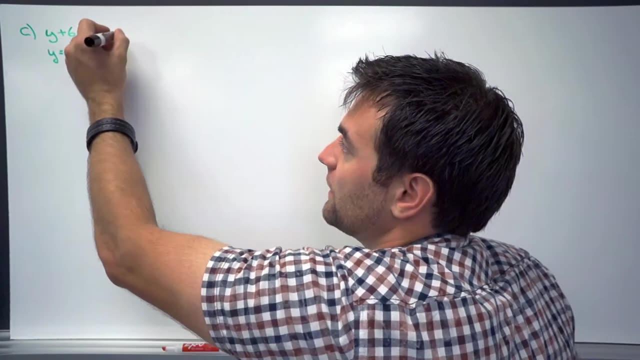 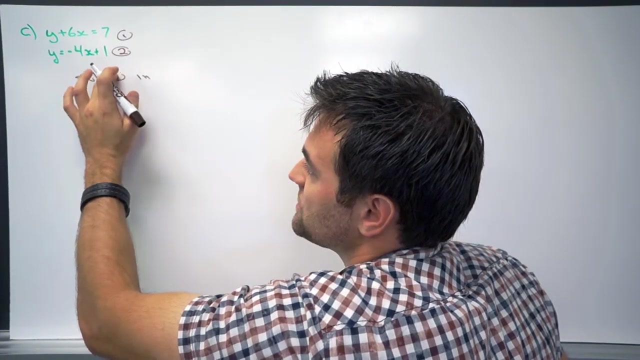 So in this case, here we have an equation that we have to sub into an equation a little bit different, but the same procedure is followed. I'm going to name these 1 and 2 and I'm going to sub equation 1 or I'm going to sub equation. 2 into equation 1.. That's y equals. so I know y is equal to negative 4x plus 1, so I'll have negative 4x plus 1 in place of the y plus 6x equals 7.. And I just subbed. 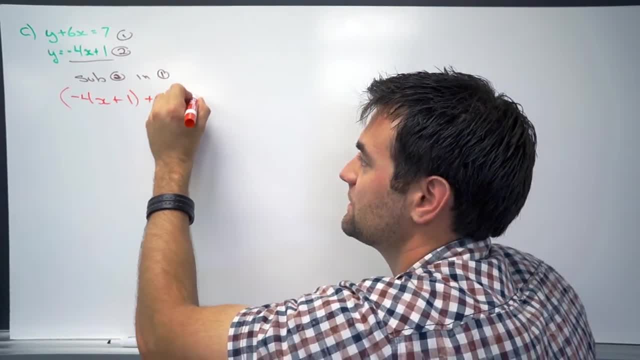 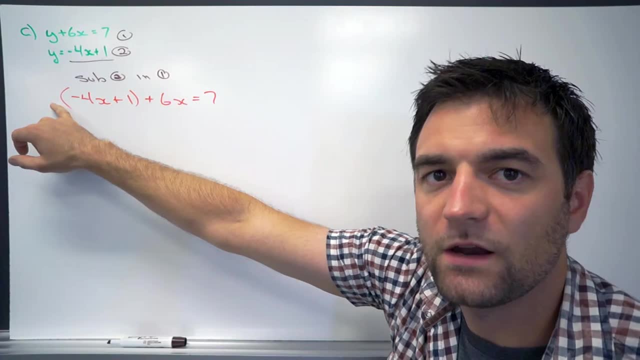 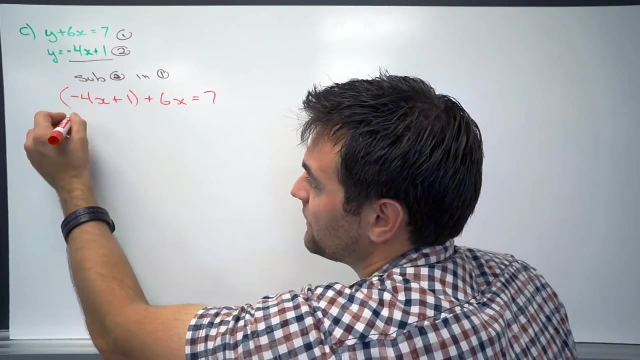 that whole equation And put it in brackets. just in case there was a number up front that I had to multiply by, I'd make sure I multiply everything through the whole equation. Now I don't need the brackets, so I can drop them And negative 4x plus 6x, that's going to give me 2x. There's. 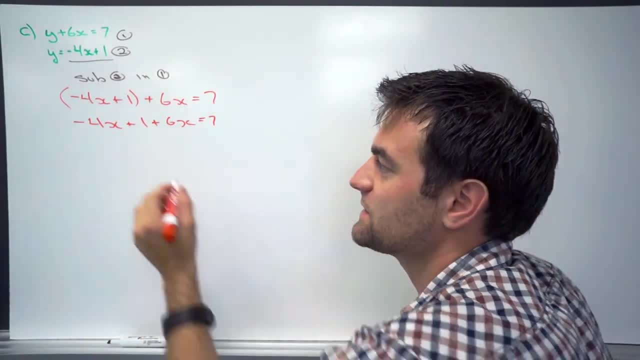 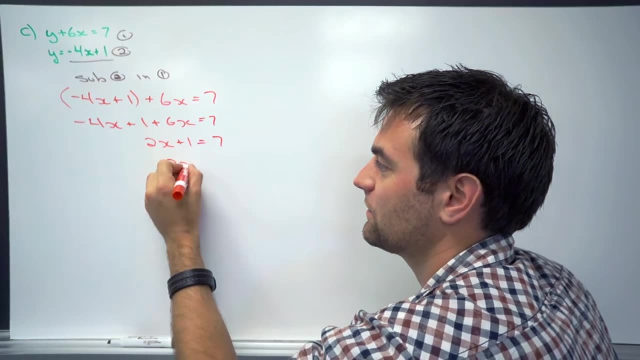 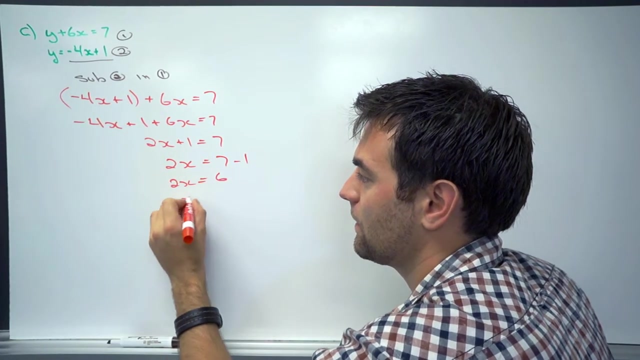 a plus 1 in there and still a 7.. Now solve this for x. I'll move the 1 over and make it subtract 1. And then I'll move the 2 over, And it'll be 6 divided by 2, which is 3.. So I found my 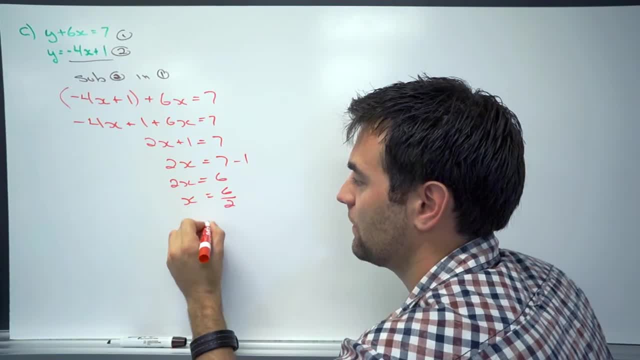 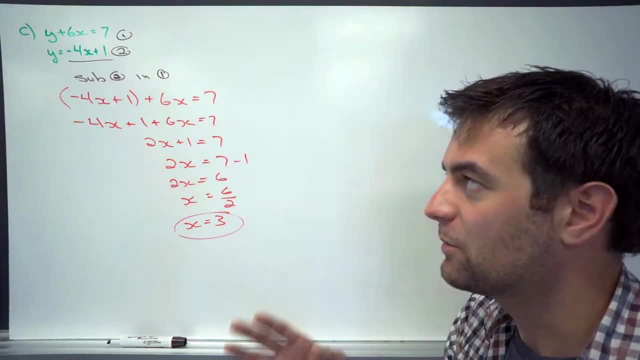 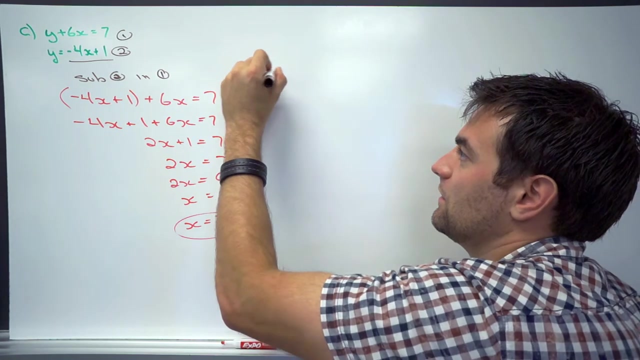 x value. Now I still need to find my y value. Remember, we're finding the point of intersection, which is two coordinates. So I have the x. I can take this now, sub x equals 3 into equation 2.. And I'm picking: